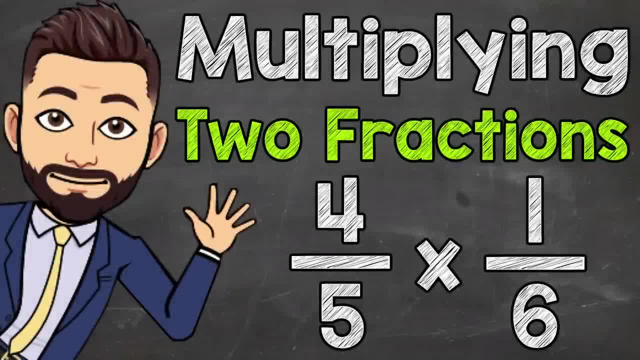 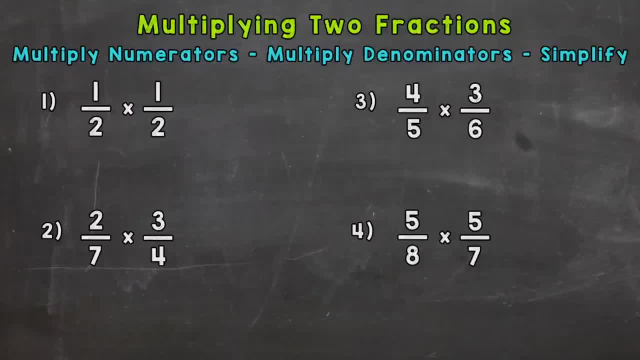 Welcome to Math with Mr J. In this video, I'm going to cover how to multiply two fractions, and we have four examples that we're going to go through together in order to get this down. Now, when it comes to multiplying fractions, the steps are at the top of the screen. We're going 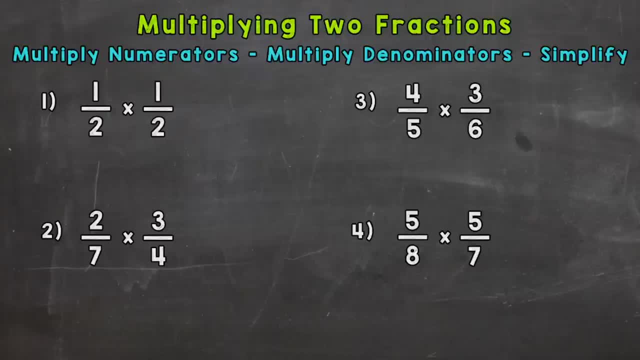 to multiply the numerators, multiply the denominators and then simplify. Multiplying fractions is actually simpler than adding or subtracting fractions, because we do not need a common denominator. So let's jump into number one here, where we have one half times one half. 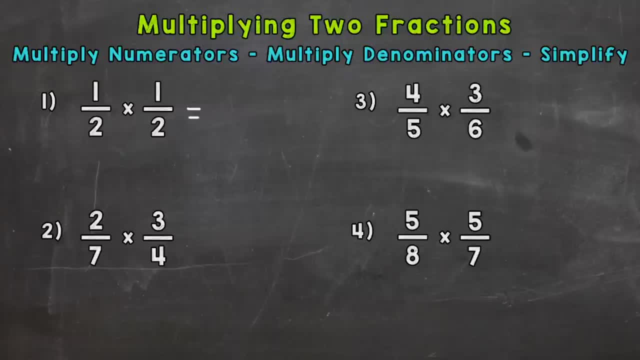 So first thing again, we need to multiply the numerators. so the top numbers One times one is one. Now the denominators, the bottom numbers Two times two is four. So one fourth is our answer and we can look to simplify. 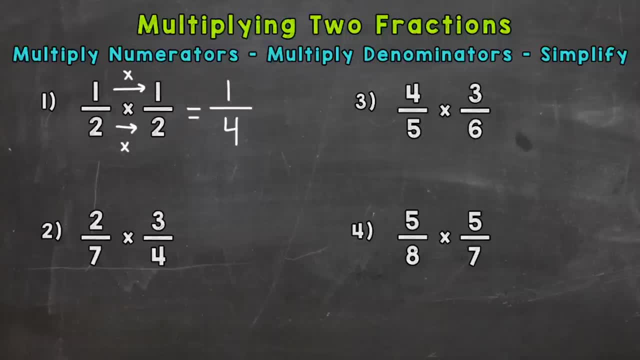 One fourth happens to be in simplest form because the only common factor between one and four is one. So this is our final answer. If you need more help with simplifying fractions, I dropped my video about that down in the description. On to number two, we have two sevenths. 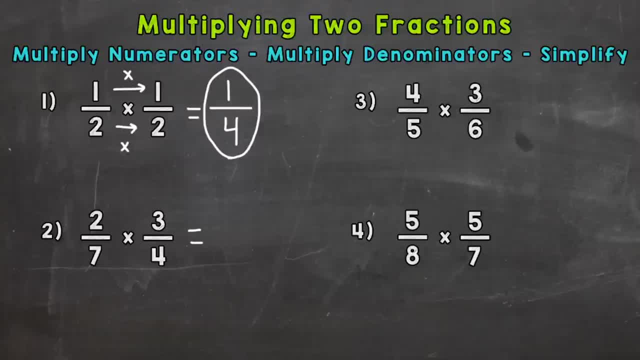 times three, fourths. So multiply our numerators. Two times three is six. Seven times four is twenty-eight. A common factor between six and twenty-eight is two, so we can divide both of these by two in order to get simplest form here: Six divided by two. 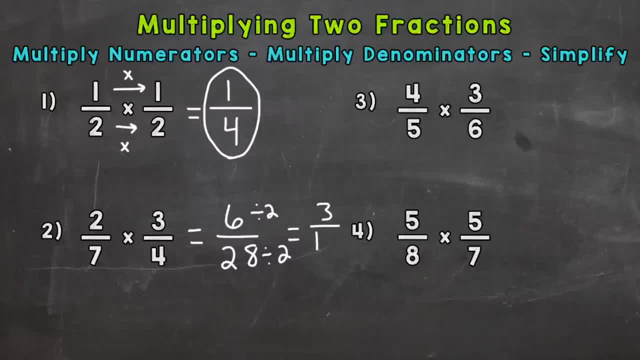 is three and twenty-eight divided by two is fourteen, So three. fourteenths is our final answer. On to number three. Four times three is twelve. Five times six is thirty, So a couple of different ways to simplify this. You can break it down in multiple steps. 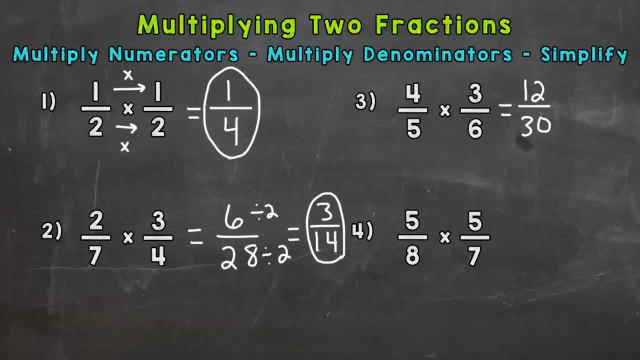 and do it in one step. So twelve divided by six and thirty divided by six would give us the simplest form of two-fifths, And what I mean by multiple steps. if we had twelve-thirtieths here, you can see that they're both even So you can divide by two, divide by two and we get six-fifteenths.